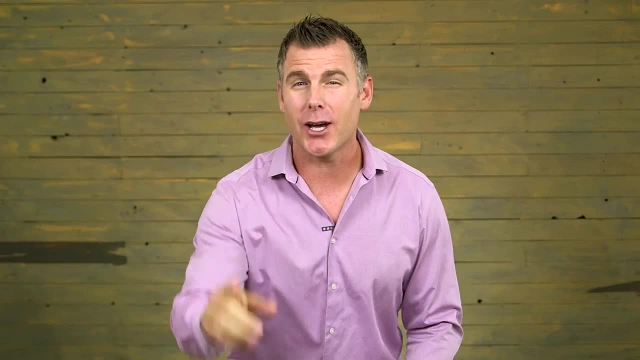 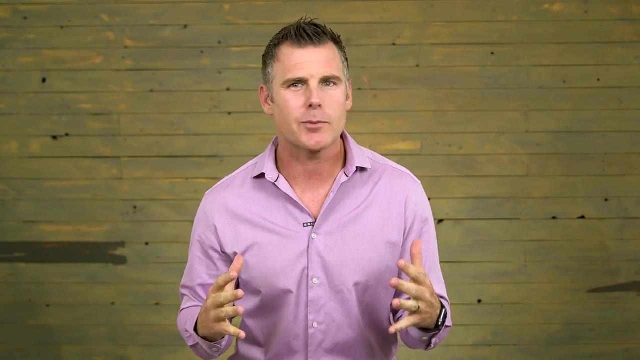 If you haven't noticed, we are in a new studio and I've got an exclusive for you today. The reason why is I'm undecided. It's a little yellow and I know this. You're probably like: well, is that supposed to be brown? 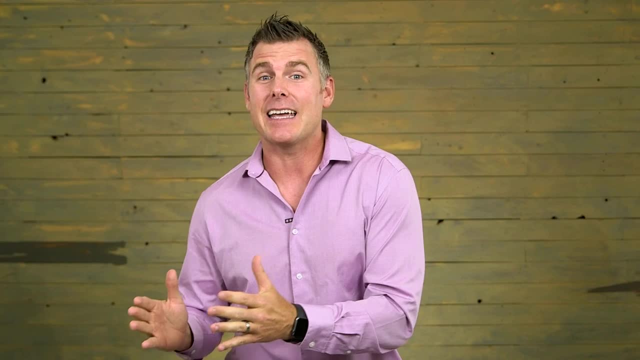 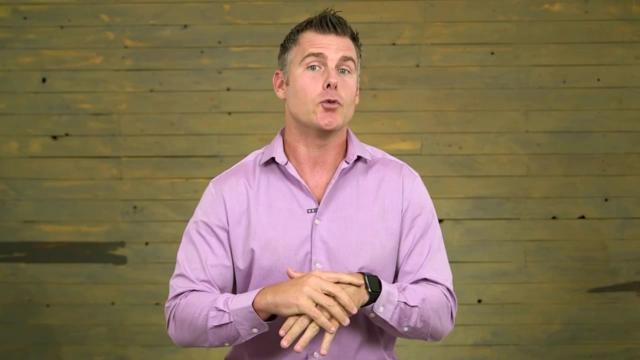 I'm gonna tell you the story to help you actually understand the lesson I wanna share with you, which is managing a project and how to go wrong. You know, if you're frustrated because you get people to build stuff for you and it's not what you want. 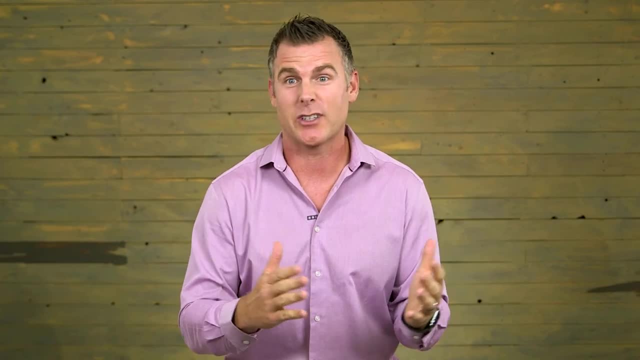 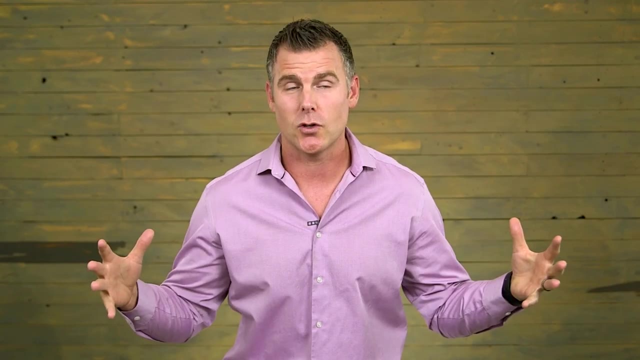 or the timelines are way longer than you had thought or proposed or even communicated to maybe your customers, or the expenses and the costs have been kind of blown out of control. I mean, I remember one time a guy called me: 1.5 million invested in a software product. 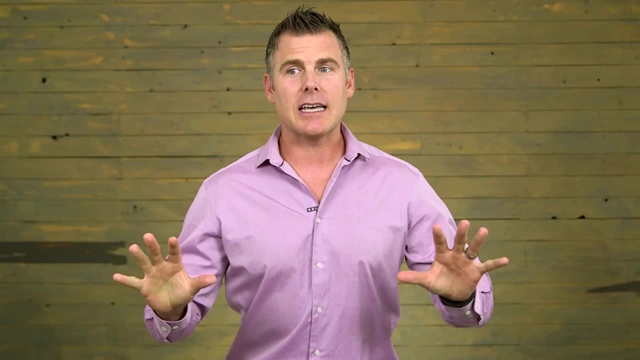 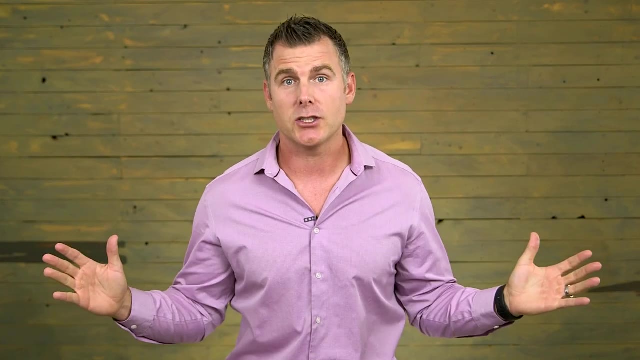 over a two year period still hadn't launched. If those things, maybe that's not as bad as that. but if you feel like you're trying to build the right product and you can't figure it out, I wanna share with you guys my strategy for managing. 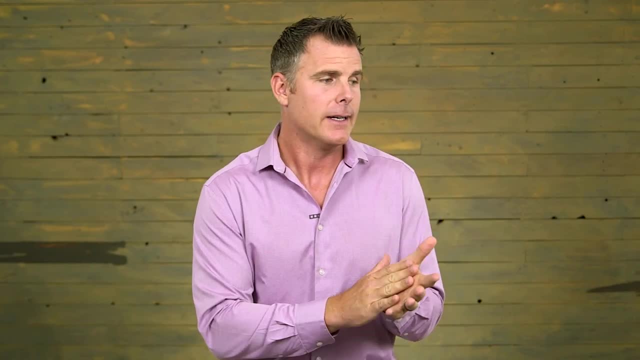 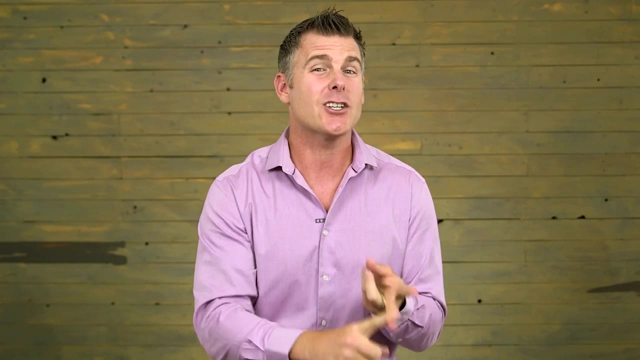 really any project, but very much specific on software. And when you do this right, the cool part is you get working product in front of a customer- Things that your customers wanted in the first place. most of waste in a company is building things for people. 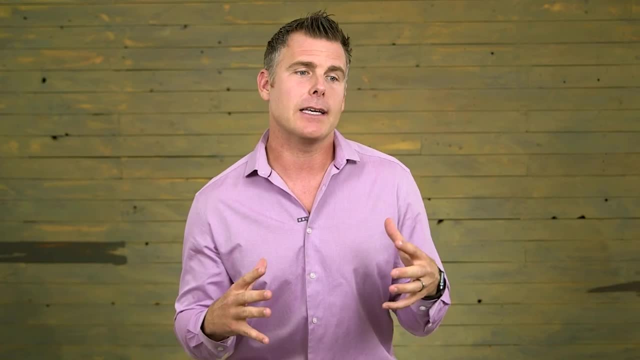 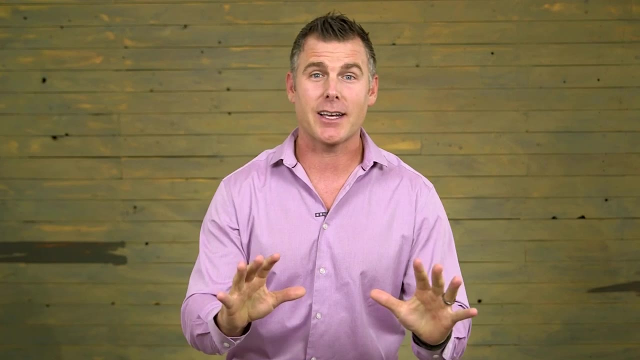 that they never wanted because you weren't listening properly, And then finally making sure that they're done on time and on budget. You know this backdrop, okay, and I'm not gonna throw Tim Tim if you watch this video. man, I really appreciate. 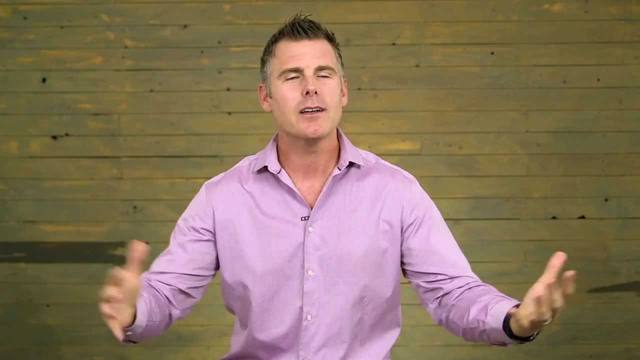 the energy and effort. I had a vision. I was like you know what We've been doing- the brick background for a while. A lot of people didn't realize it was real. You know, many times I've gone back, knocked on it. 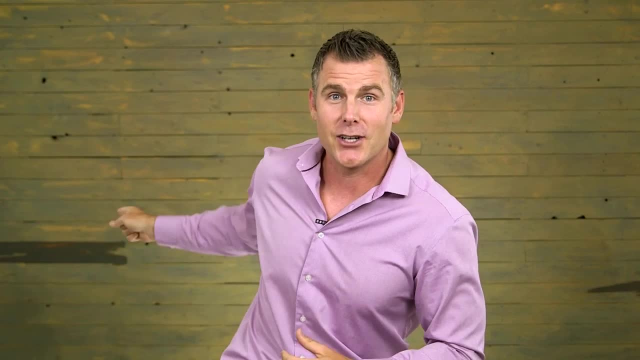 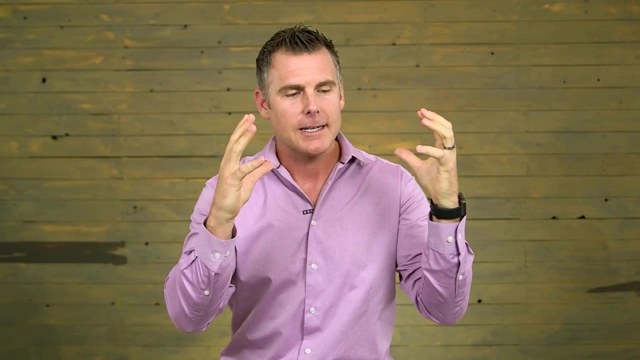 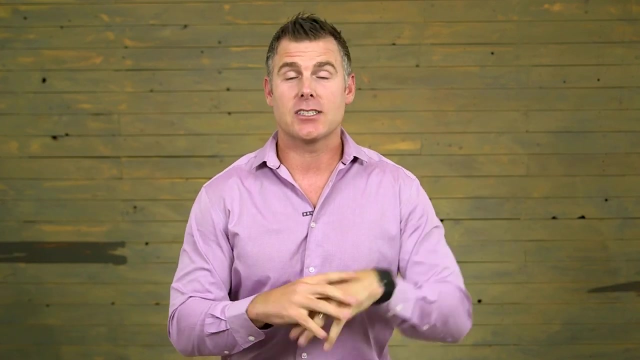 This is hopefully definitely real, because you can see the, the dark spot, stain, the knots, the holes. It was like I had this vision for kind of like this rustic wood type of organic thing, and not that we didn't achieve that, I just think the color was off and it showed up. 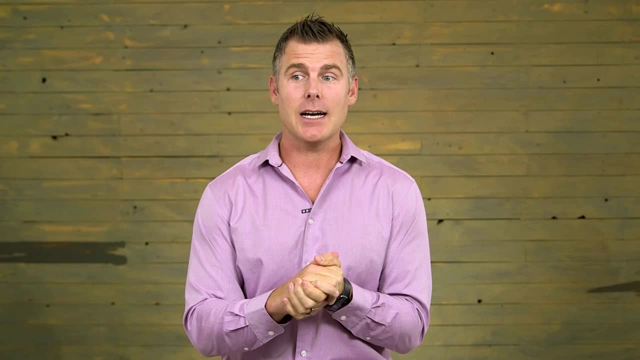 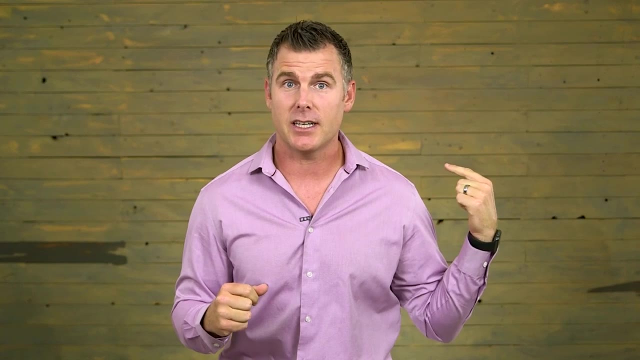 and I wanted to shoot some videos. so here's the deal. I want to share with you what I shared with Tim, because I hired Tim to do it. We had to engineer this thing. I mean it's heavy, It's got aluminum frame. 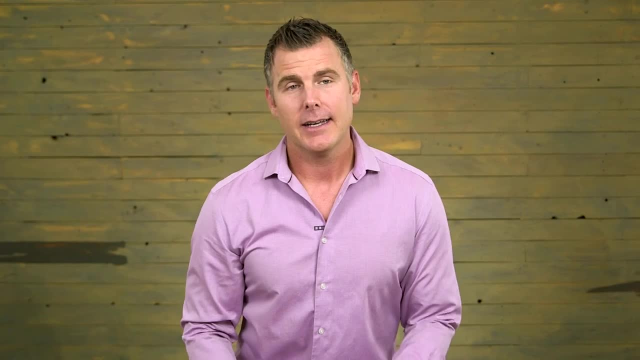 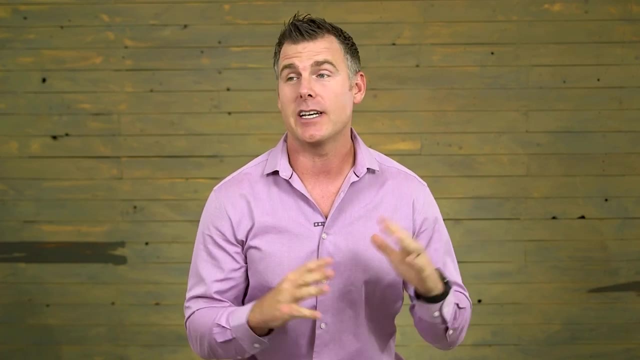 It's actually a quite cool piece of studio gear, but I really learned how to manage projects back when I was 21.. I got a job that I should have never got: managing a team of engineers at a company called Syncrude, getting paid way more. 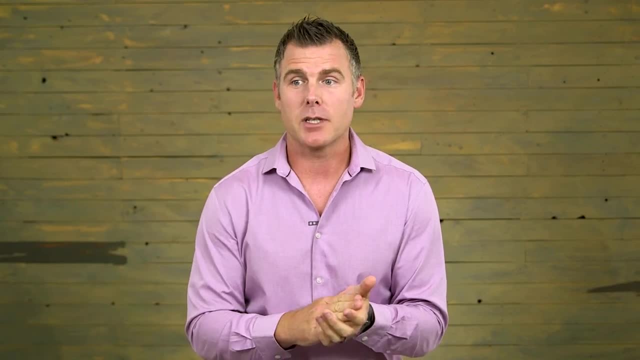 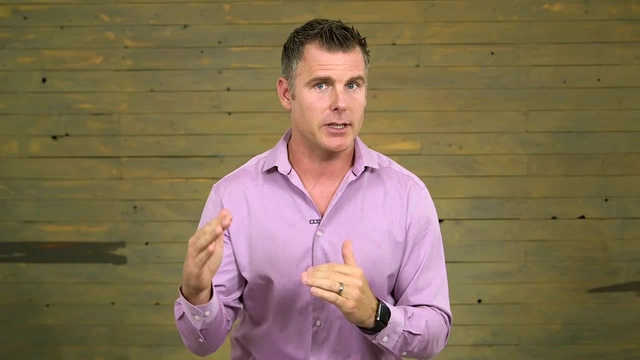 money than I probably should have been getting paid and my boss pretty much pulled me aside because we interviewed over the phone. he looked up my resume. Maybe he didn't do the math on how old I must have been based on when I went, You know, graduated and stuff and I was a contractor and he 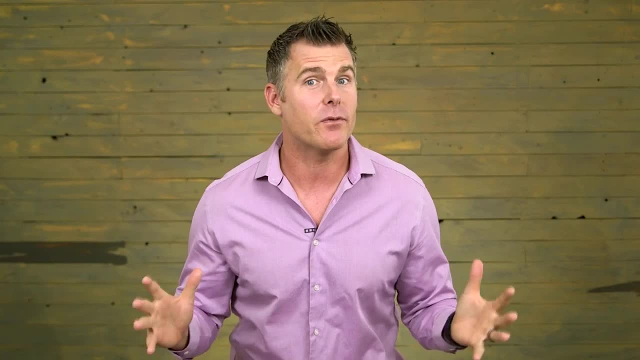 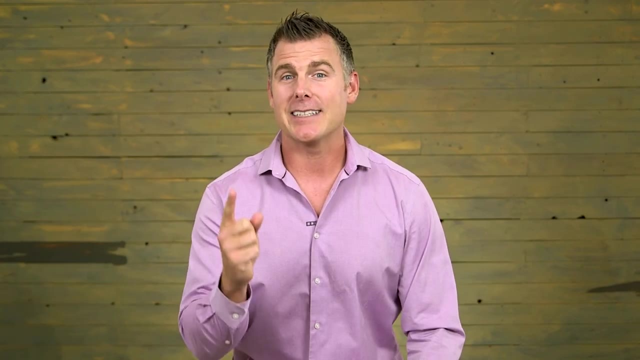 pretty much said you have two weeks to figure this out, and I didn't really know what figure this out means, but I did. what I hope anybody would do in my position is: I went to the library and I got a library card and I started buying books. 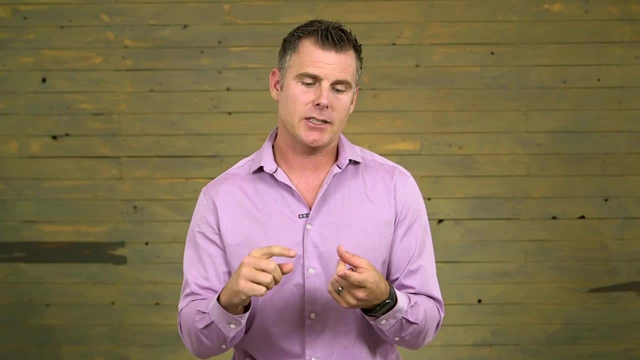 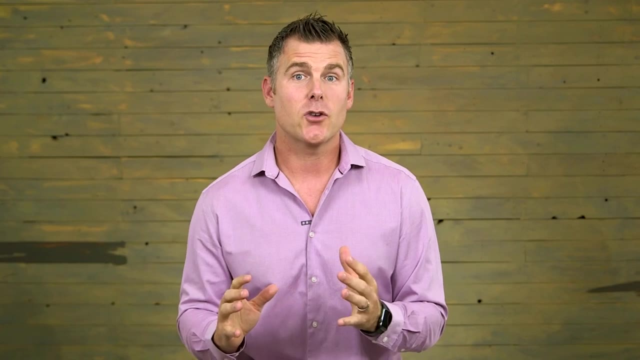 I was gonna be responsible for about a team of 30 people, so I needed to understand how to manage those people, how to lead them, how to set expectations, how to interact with vendors. so I rented, rented, borrowed. I mean most of you guys are laughing. 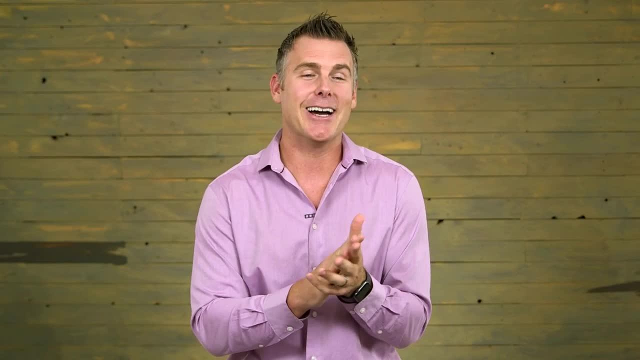 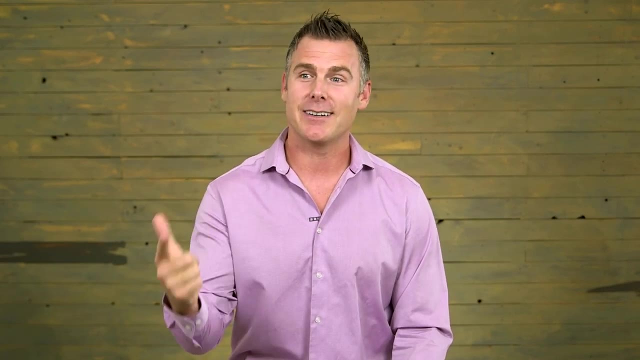 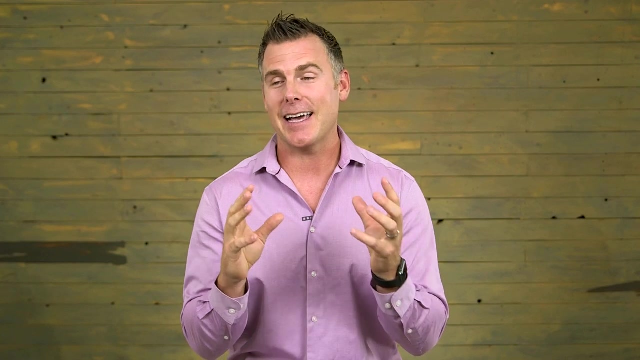 You've probably never been to a library. I guys, isn't that funny. We live in a world where you've maybe never been to a library, and I got books on project management, I got books on technical architecture, I got books on understanding the world of consulting, and that's. 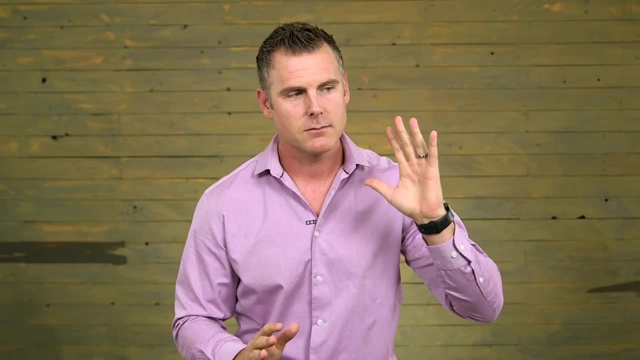 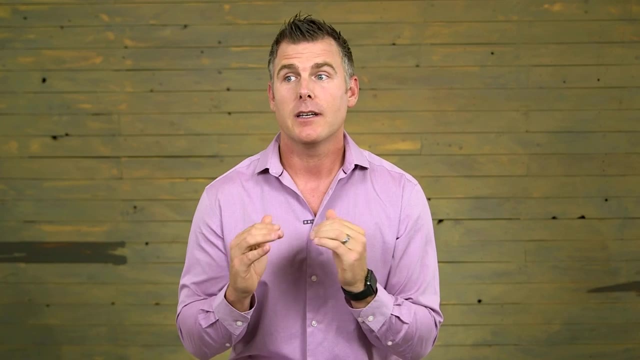 where I learned Gantt charts. I'm still undecided how I feel about them, but that'll be for another video. and it was through that experience at 21 to 23 where I really refined my approach. I got books on technical architecture. I'm still undecided how I feel about them, but that's where I 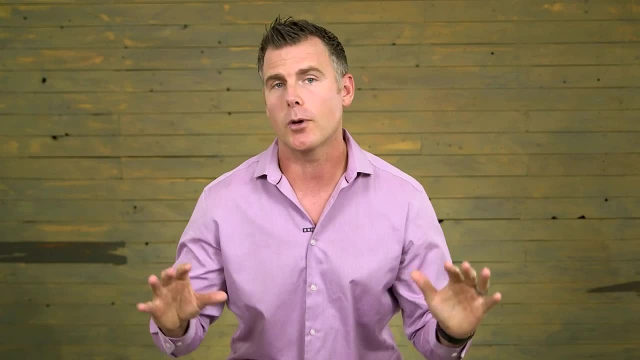 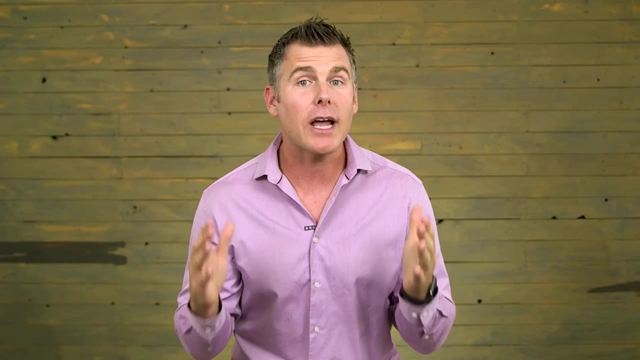 really refined my approach to managing projects, and what I wanna share with you today is the four key areas that I think are super important. Number one is time blocking. When you build something new, you need to set the constraint. If you don't have a constraint, then anything is possible. 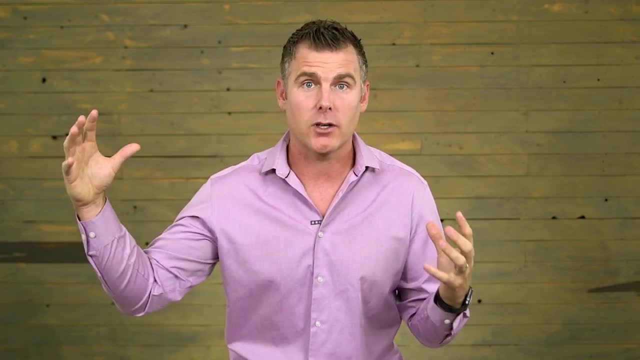 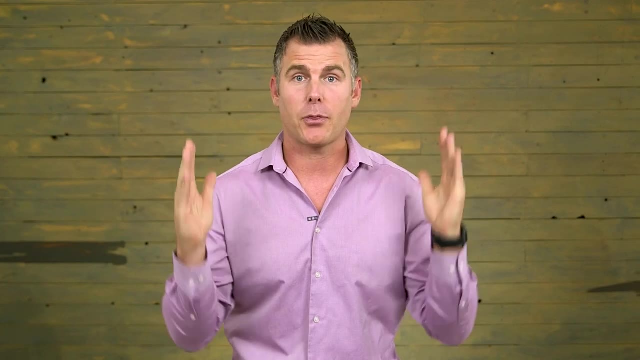 The scope for what you wanna build can expand way beyond what you could possibly do with the resources you have, and it's super important to actually like say okay from a time point of view, we've got three months and we're gonna build this. If you're into agile development, which I highly suggest, typically you're doing kind of a six week product kind of road map with two week iterations and sprints. but regardless, no matter if you're starting off from scratch in your first time building software or you've got a team. 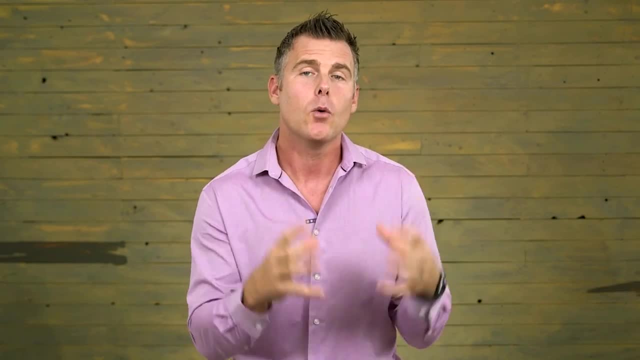 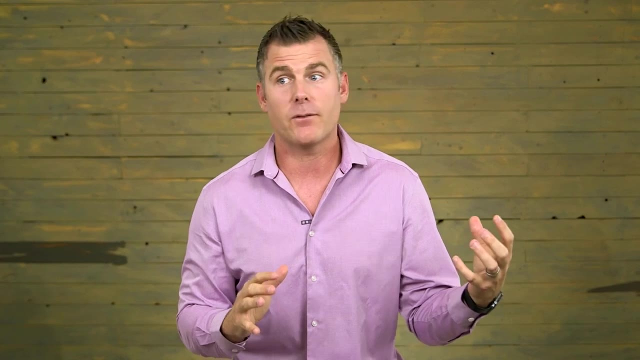 you want to set a cadence for time, blocking what gets built in that time frame. so that's one Number two: you wanna make sure that you define the outcome, and for me this is really from the user's point of view: Most of the features you're gonna build that are not paying. 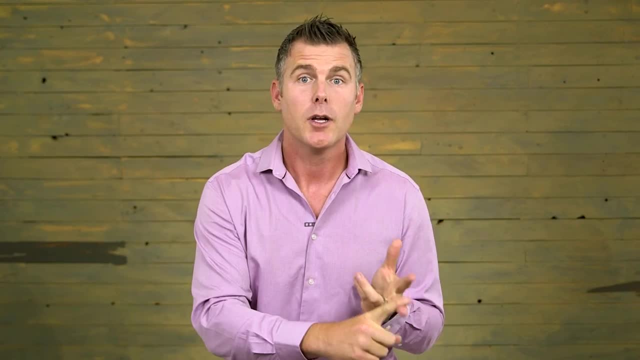 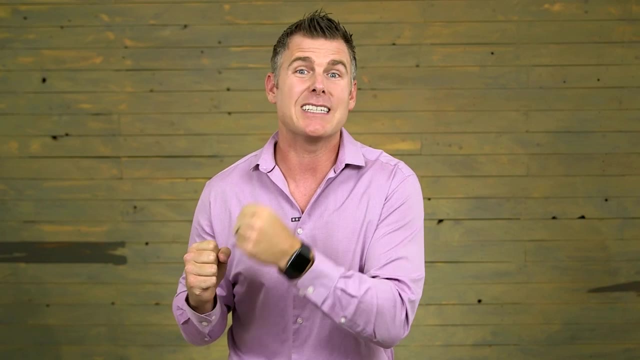 down code debt and kind of fixing things. performance, that kind of stuff or fixing bugs are gonna be focused on the user and really trying to help them achieve what's called the desired outcome, and the way you do that is user story, so making sure that you have a defined outcome. 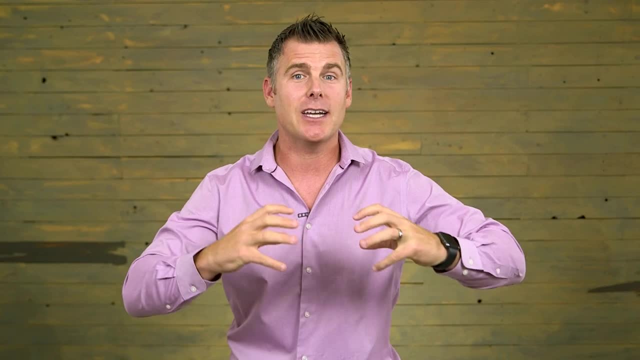 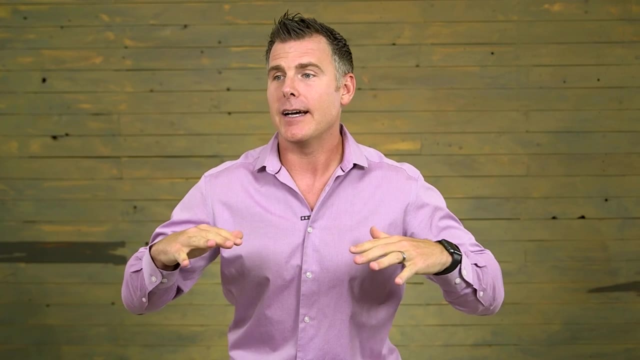 for what you wanna have done. I wanted this built and we talked about it and I was like you know, it's gotta have handles because it's a big, heavy piece of gear and it rolls around and it's in a studio and there was all these things and one of the things that I felt 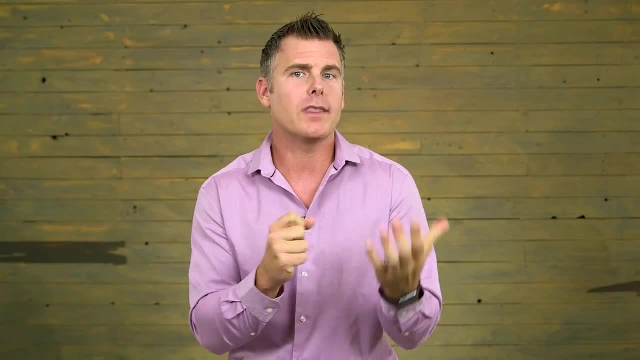 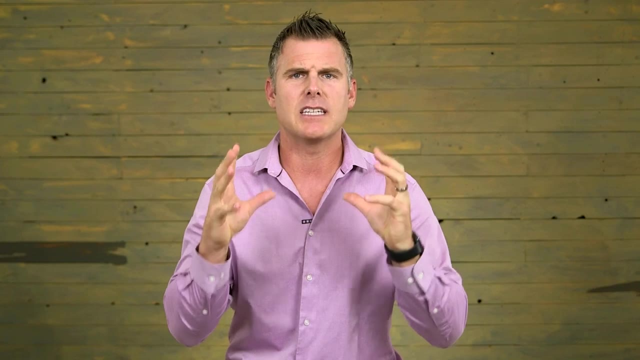 wasn't really captured was the outcome goals. okay, What the specs were. We talked about it, you know, but it was never really written down, drawn out and really like, okay, this is what I want you to do. And look, everybody has a different approach for managing. 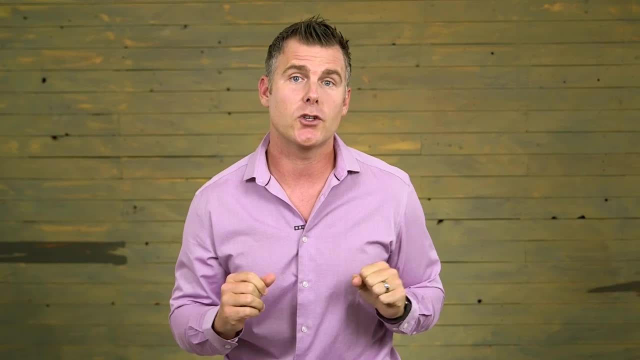 their stuff, but when I hire and delegate this to people, I'm just gonna trust that they're gonna do it the way that works for them. This is just some feedback and thoughts on how it could've went better. So time block was there. 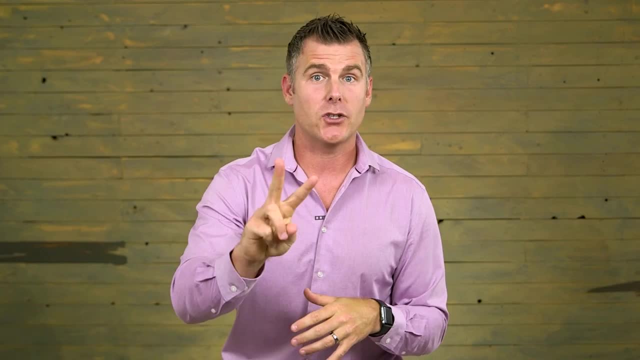 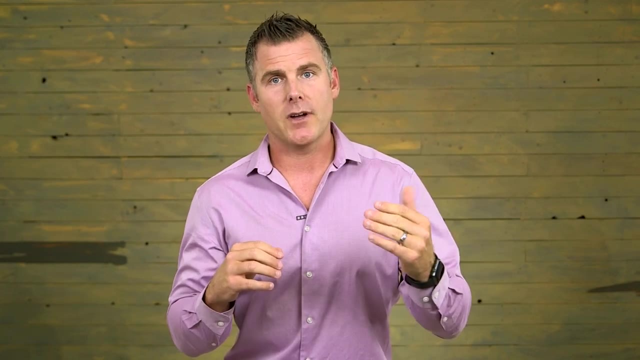 I had a date that I needed it delivered by and we were late by two days, and I'll tell you why. because it's number one, number four in this video, but it was really about making sure that the outcome goals are well defined. Number three is you need to make sure that you prototype along. 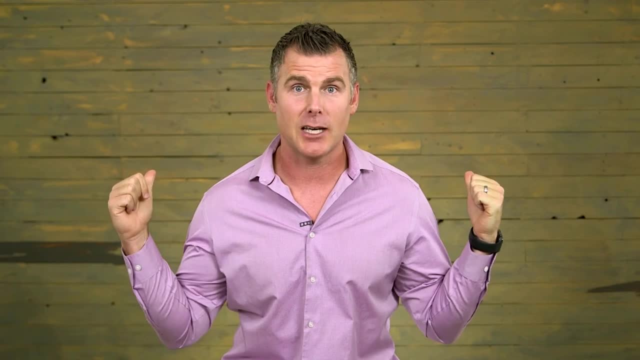 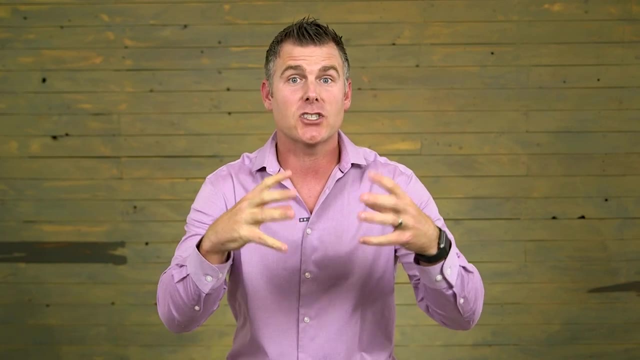 the way. okay, And what happens is- and this is an example- is the stain, the color: instead of coming in yellow, could've came in on the brown tone that we had actually like screenshotted and sent across. but the reason why is it was. 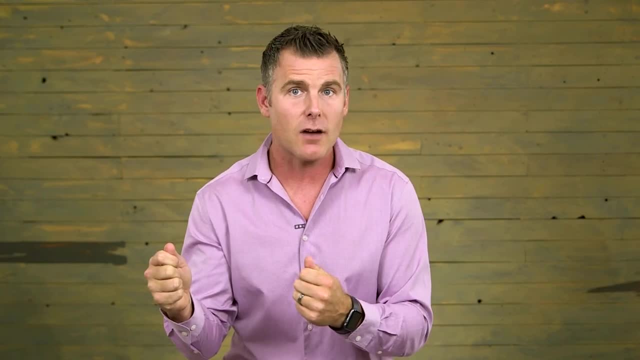 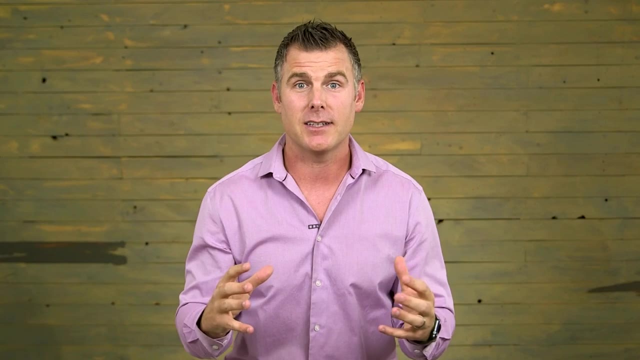 never tested right. It wasn't something like- and many times when you're building software, you communicate the specific applications using words, text, a document and I can't tell you, but like if I wrote a paragraph of an outcome I wanted and we 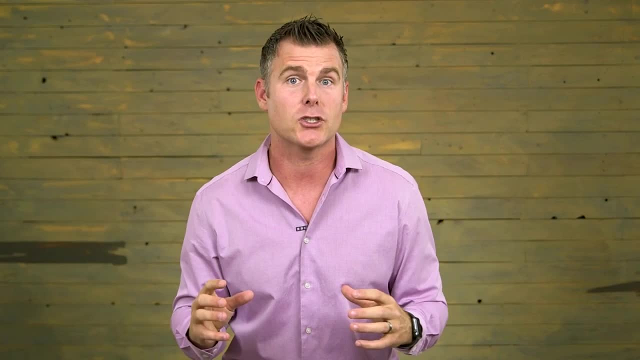 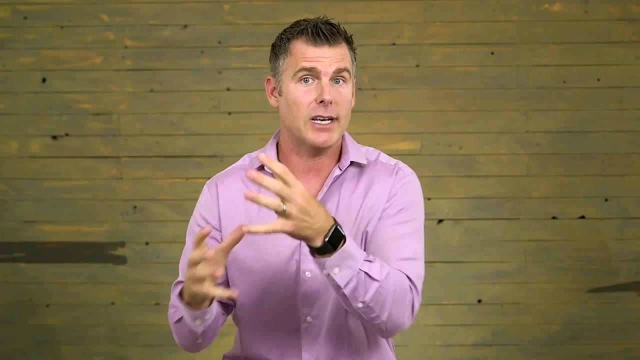 had two different people read that paragraph and kind of build towards what they think or how it should work. we're gonna have two different experiences, So to me it's all about prototyping the user experience, so it's called the UX- how it interacts. 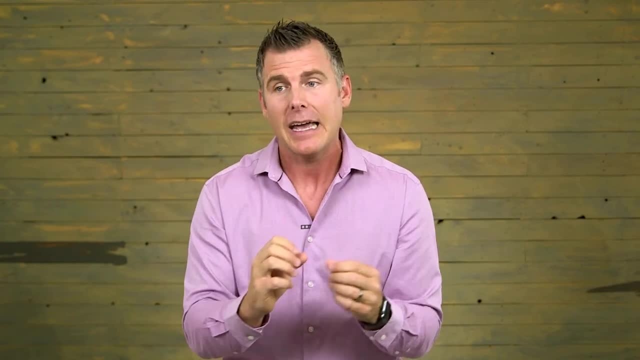 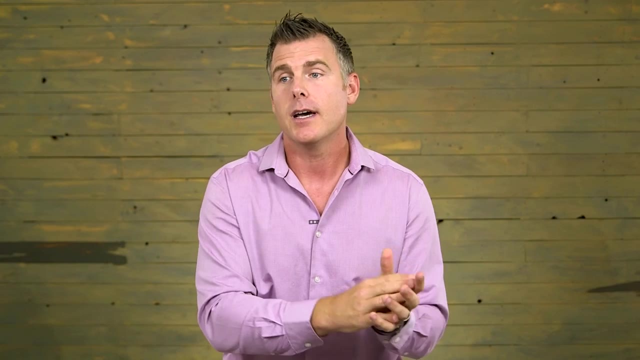 how the feature works, because there are a hundred different ways you can implement something, and also the UI, or the visual design. you know, how do you want the colors to look? how should the buttons be stylized? what layout and spacing should you use? and I think that 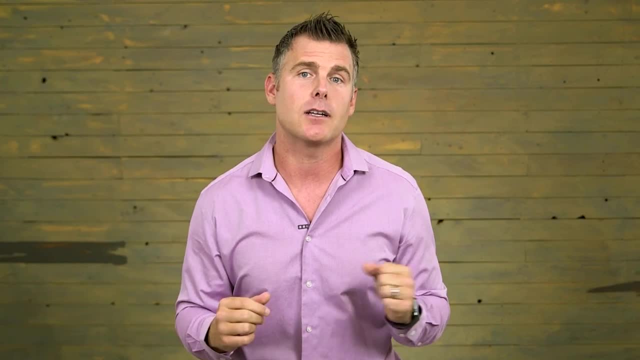 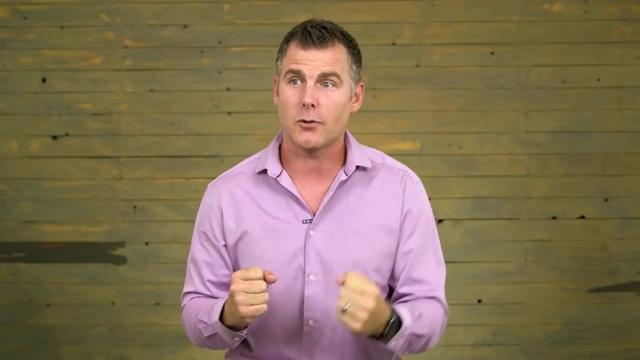 regardless of what you're gonna build at the end of the day. if there's elements in there that are unknown, you need to prototype. You can do that through a designer's mock-ups. you can do that through clickable prototypes using Keynote or UX pin or Balsamiq or whatever tools. 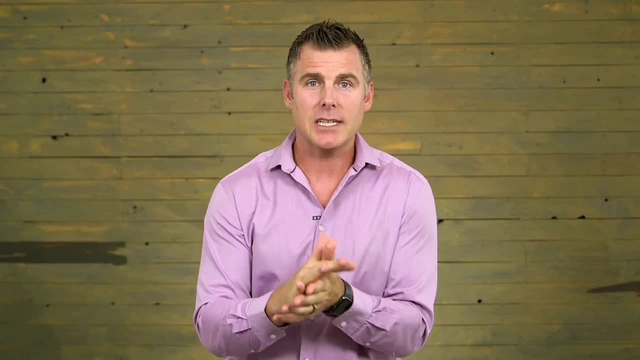 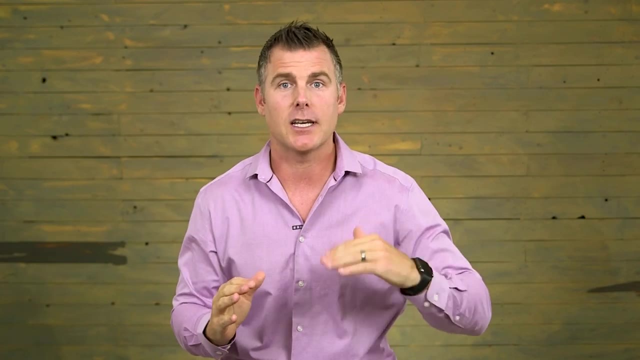 It is very important to prototype. so that's number three. Four is you need to make sure- and this is what happened- is, if there's dependencies amongst the project right, Other areas, Other business units, Other people, that you communicate with them early and 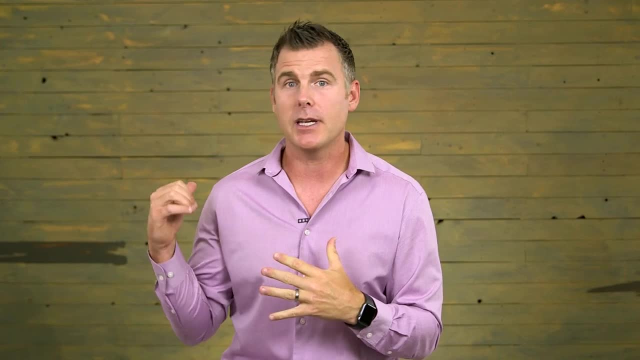 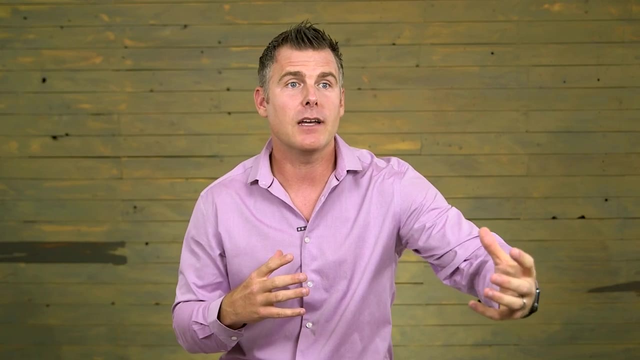 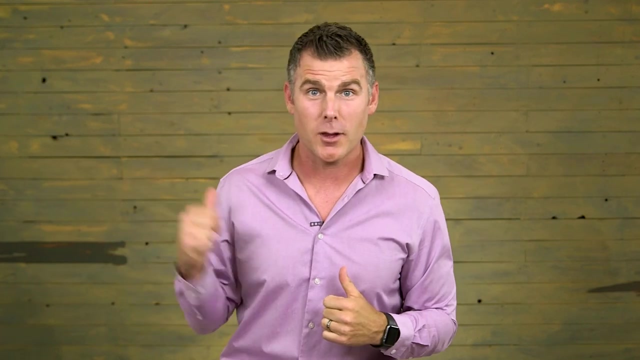 then often, especially if you own the project. So what happened here is we had to work with a contract company to do an aluminum frame and communicate those specs, but the timelines were never asked for and or committed from that person. The other thing is the custom stain for the backdrop was never. 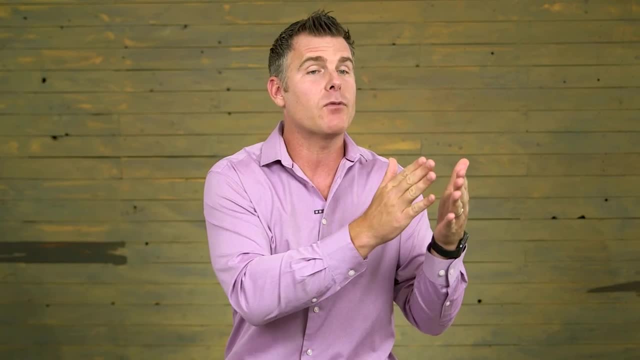 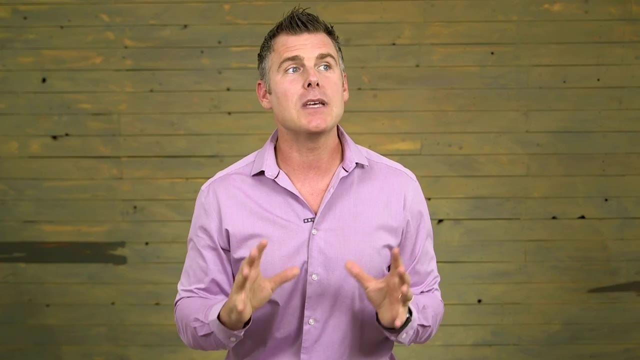 tested early in the process of the project so that if there was a discrepancy in color because there's a fixed timeline, that we could have fixed that early and get that resolved. That, to me, is probably the number one thing that every founder gets wrong is when you start a new project, and this 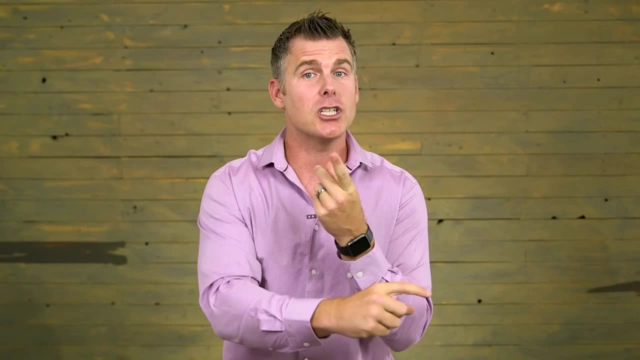 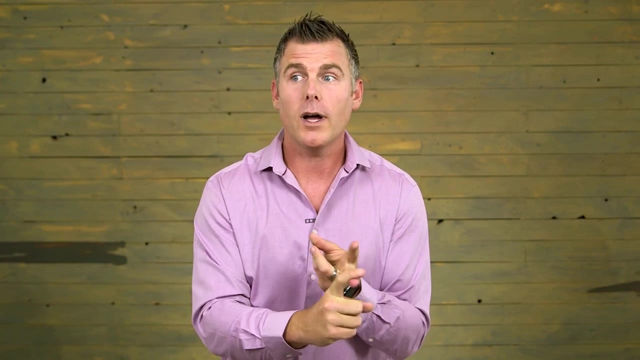 usually comes from three key areas in your business: The technology that you might assume is gonna work. so maybe that's an integration, it's an API, it's your own code technology. Second one is marketing. What are the dependencies once you build this, that marketing? 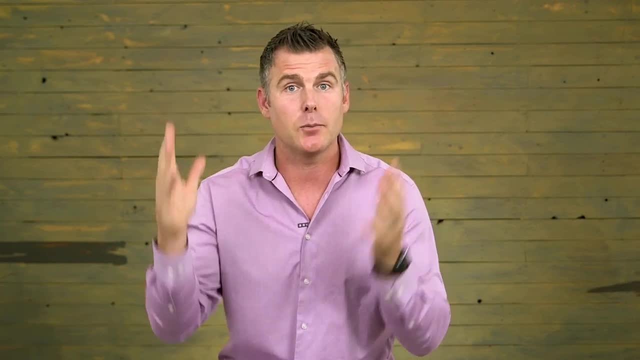 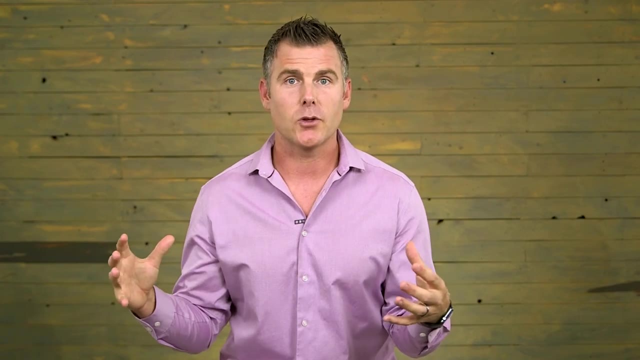 needs support on. So maybe they gotta put a campaign together. they need to put a new features section, they need to add it to the pricing page. so there's marketing dependencies And then finally operations. So you think about in your business. there's like 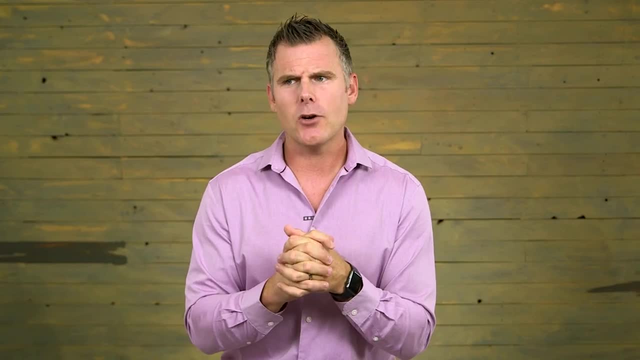 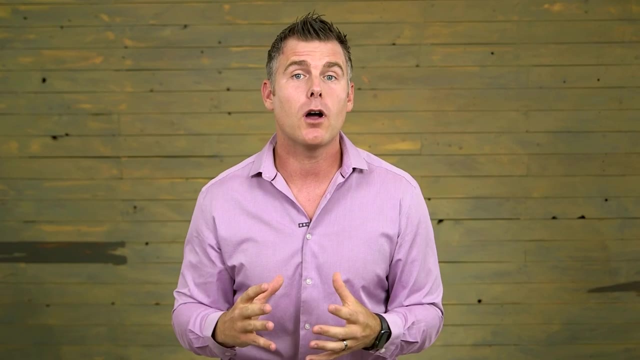 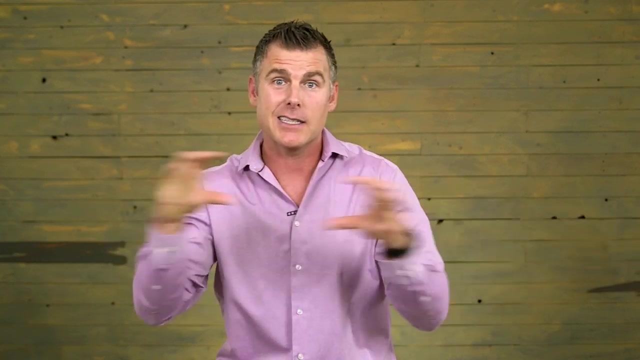 administrative support or you know it could be billing or whatever it is, but there's an operations component and those three areas are dependencies on the overall project that need to be communicated, need to be understood and, if there's legal or anything else that has to provide feedback into the